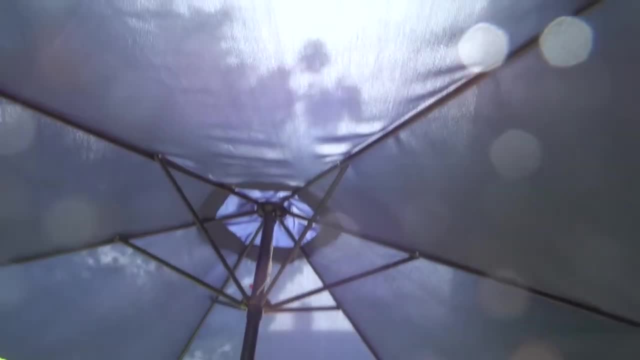 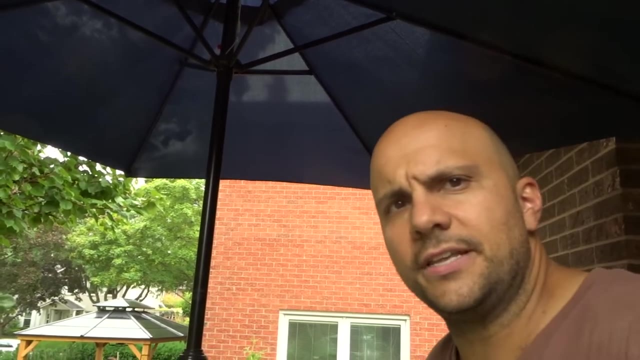 is the patio umbrella in my backyard. You can see right here I have it fully expanded and what I'm going to do is I'm actually going to get in front of the camera over here and explain what you have to do. So, essentially, when you want to measure a patio umbrella, you want to measure the entire. 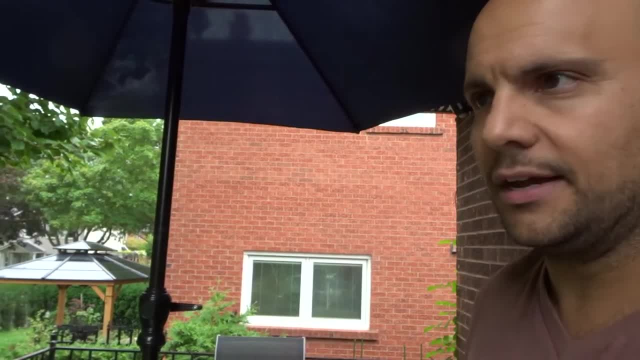 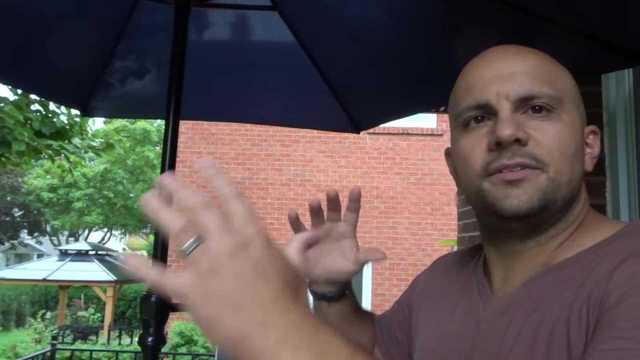 distance from one end to the other. Now I'm assuming your patio umbrella is not a rectangular shape or anything like that, because if it's a rectangular one, something that's sort of asymmetrical, then you're going to have to take some additional steps to measure both directions. 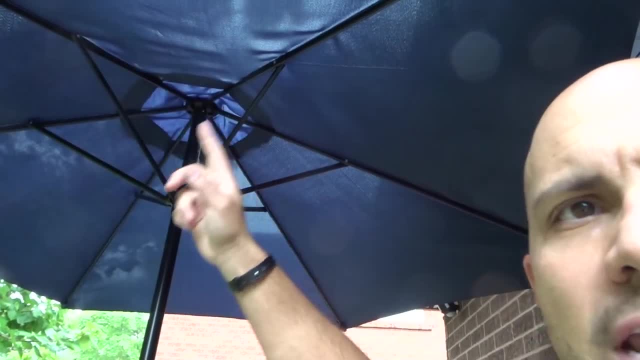 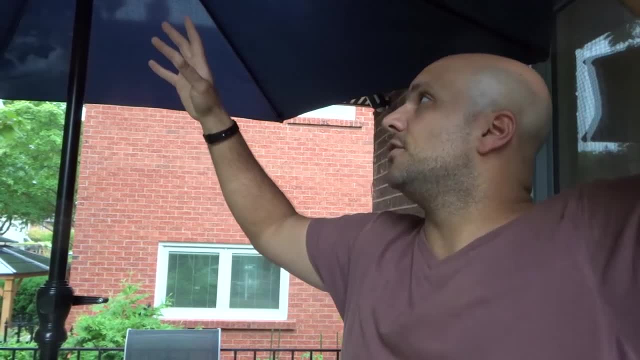 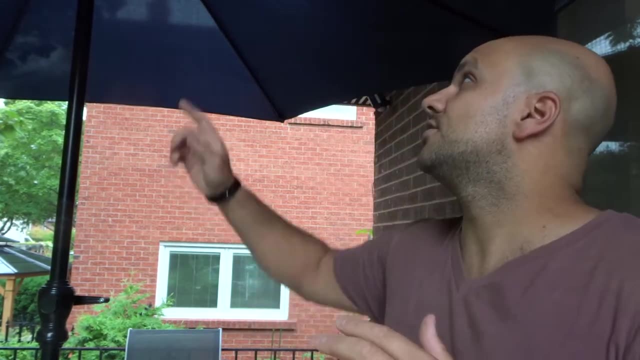 go and measure from one side to the other, But it's kind of difficult because the umbrella isn't perfectly flat, it's on an angle. So the easiest thing, the the easiest way and the best thing that you can do is to actually just go and get your measuring tape and you want to measure from the. 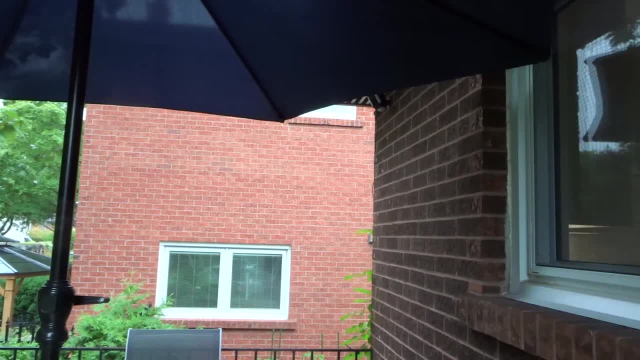 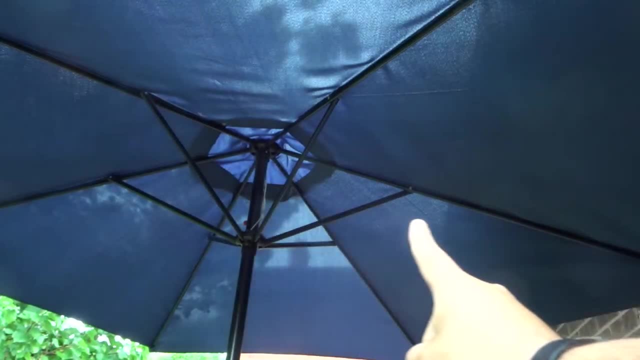 middle portion to one of the edges. So let me step behind you and show you exactly what I'm talking about, So you can see. I'm going to raise the camera up. You essentially want to measure from that middle pole all the way to one of the edges, and then you're going to take that number. 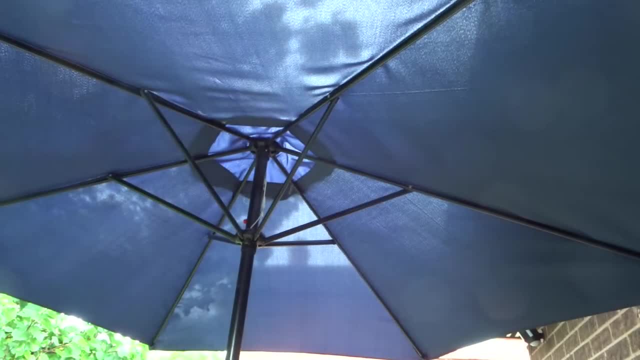 that distance and you're going to double it and that's going to give you that distance. So you're going to double it and that's going to give you your patio umbrella measurement. So what I'm going to do. now let's aim this upward. I'll try and show you exactly what I'm going to do. So there we go. 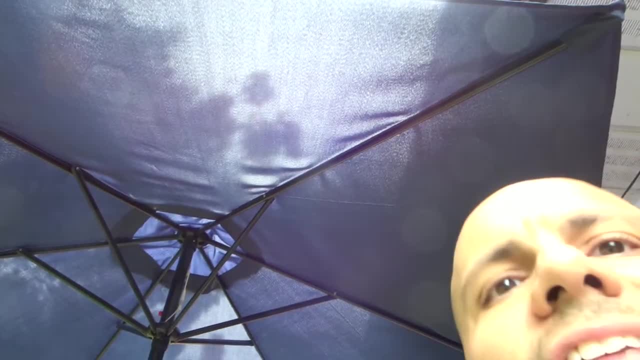 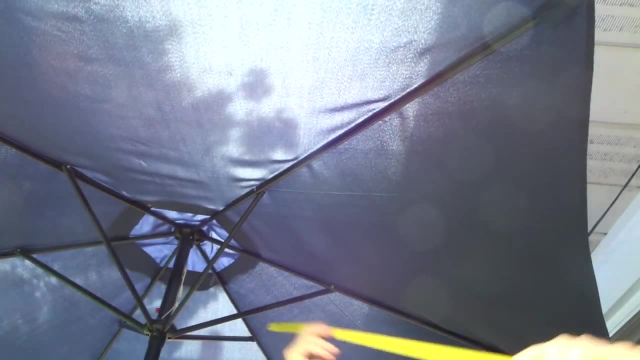 Flip my screen so I can see exactly what you are seeing. I can't exactly see because of the glare, but I'm going to just make sure I'm measuring the right pole that you can see right here. So, essentially, I'm going to take my measuring tape, I'm going to place it in the middle, okay, and I'm going to measure to the end over here, okay, and the number that I'm getting is four feet. So essentially, the distance of this patio umbrella from the center to the edge of one of the poles is four feet. So if I was going to go get a replacement patio umbrella, I would want one with an eight foot. canopy, because four feet times two is going to be eight feet long and that's honestly, it's that simple. A lot of people think when you measure a patio umbrella, you're measuring like the distance upwards, like that right, you know the height of it. but that's not usually the case What you're going. 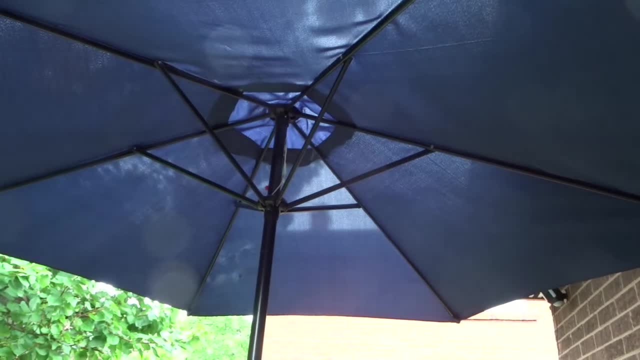 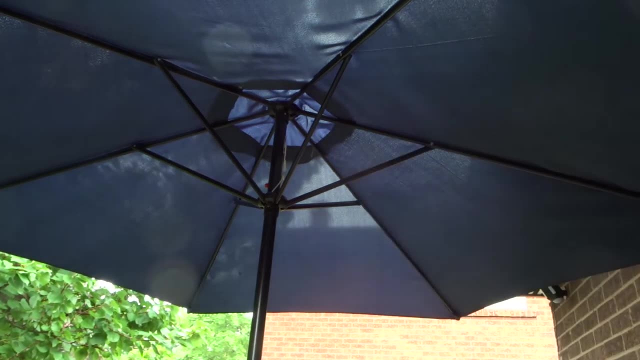 to be measuring for the most part is going to be the canopy length. So just take half of the canopy length and then multiply by two, and in this case, half was four feet. so my total canopy that I'm going to be looking for is going to be eight feet, and that is essentially it. Honestly, it's actually 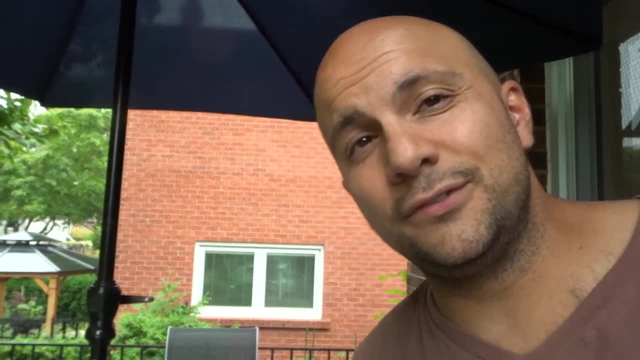 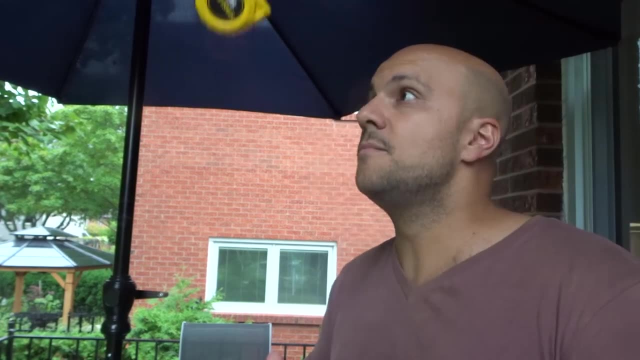 really easy to do and you can get the patio umbrella that you're looking for if you use this method. And that's it. if you like this video, please be sure to give it a thumbs up. let me know what you think down below as a comment and, of course, be sure to subscribe for more great. 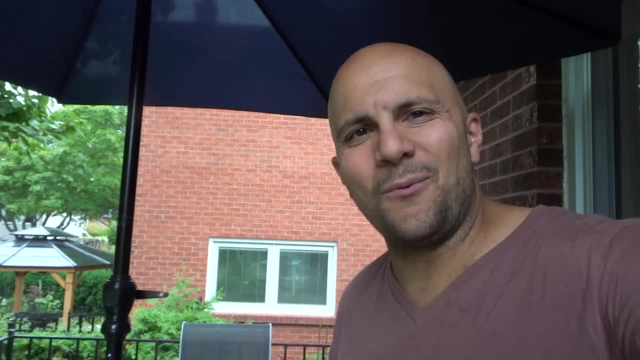 videos just like this one, And that's all I have for you today. Thanks for watching. 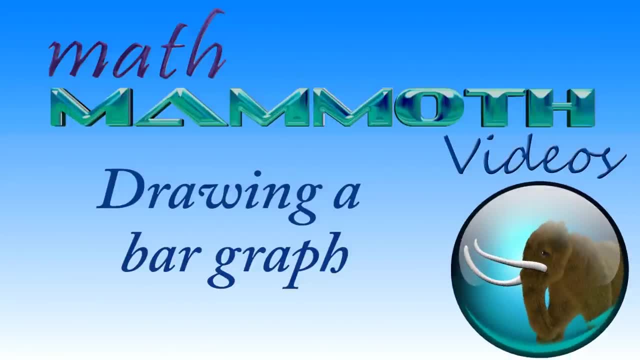 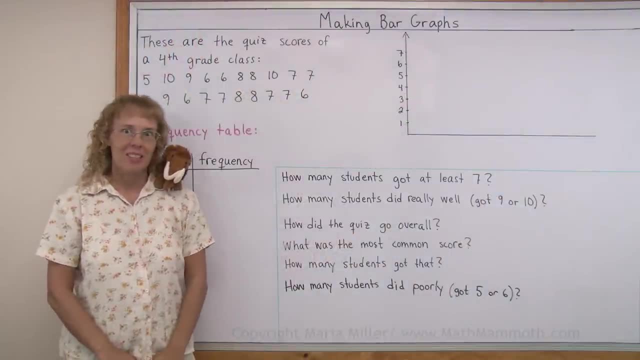 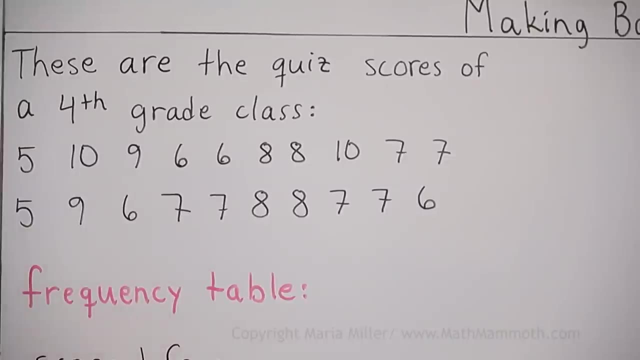 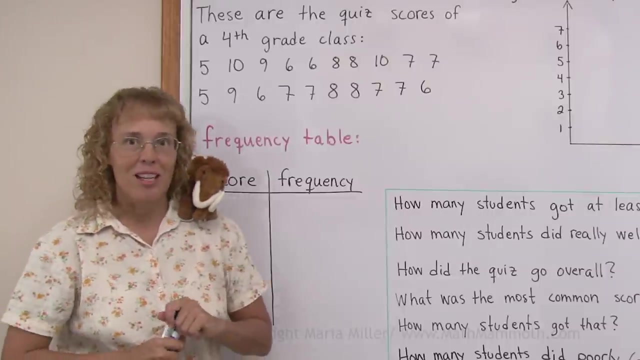 Hello, my name is Maria and this is Matthew, my mascot. In this lesson we are studying how to make a bar graph, And here I have some data. These are the quiz scores of a 4th grade class. What's that, Matthew? Oh, he's saying it was a math quiz, right? Yeah, we can think. 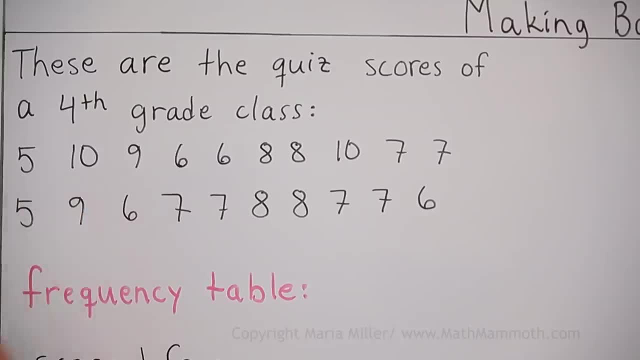 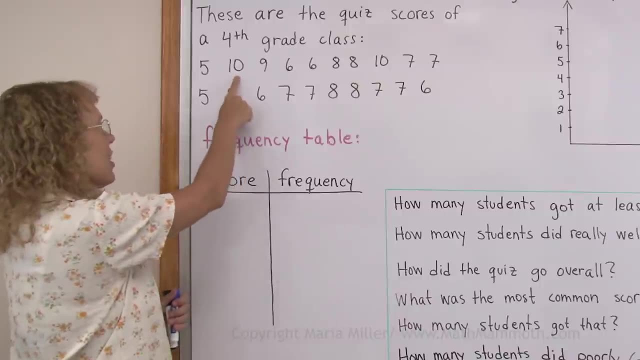 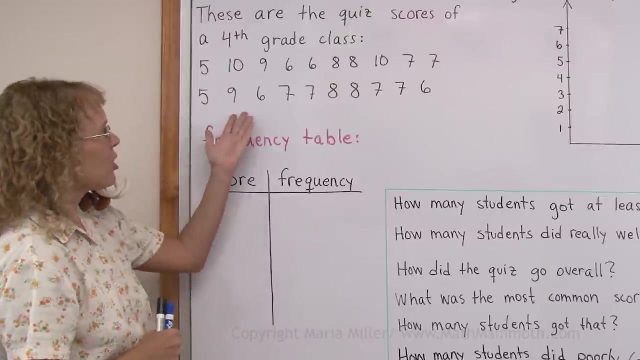 of it as a math quiz And these are the scores. So, for example, 5 means that one student got 5 in the quiz, Another student got 10.. A third student got 9, and so on, And so we want to make a bar graph out of this information. here We have to start out by making something called. 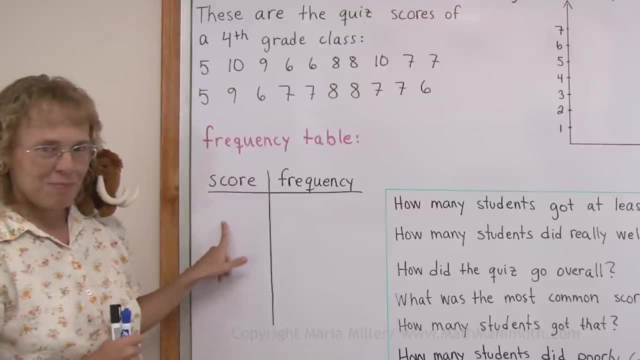 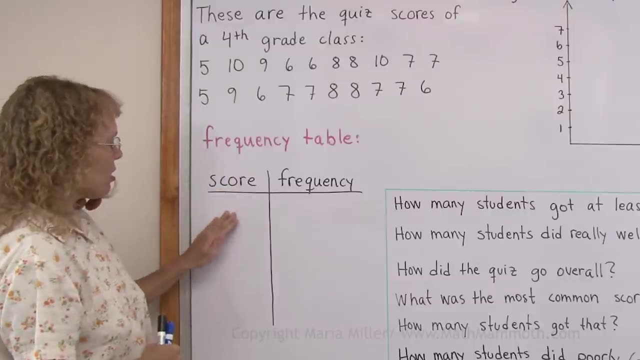 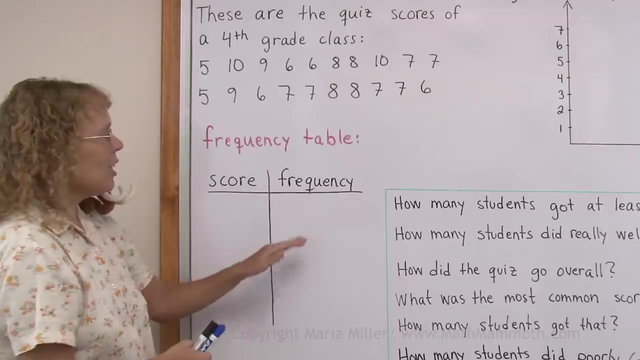 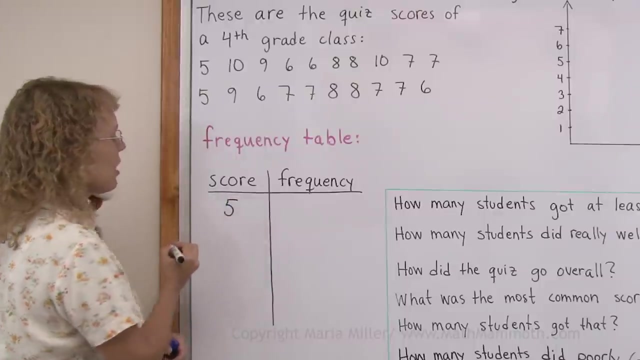 a frequency table. I'm going to make it here. I'm going to fill it in here. Frequency means how often Okay Scores are the possible scores in the quiz, Such as, you know, 5 points, 6 points and so on, And how often or how many students got that, So 5.. Some students got 5 points. 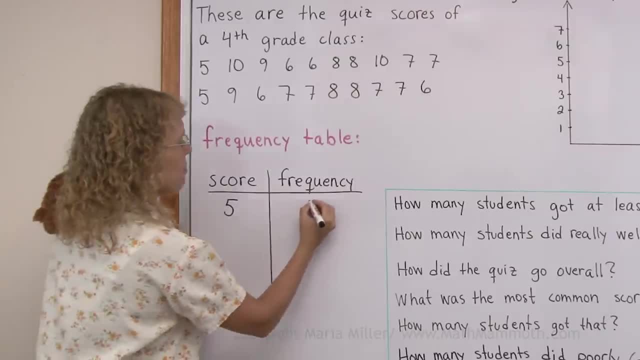 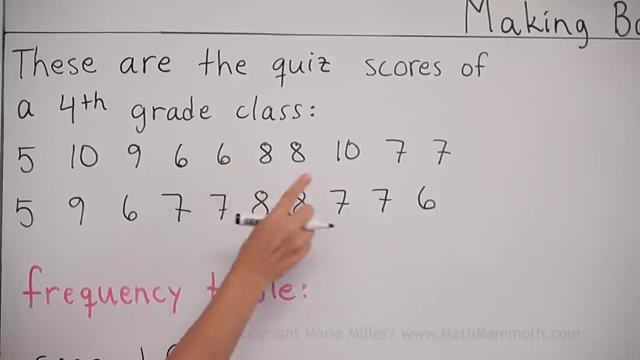 But how many 2 students, That's how often, or how many The frequency, And then 6.. We need to count here. There's 1, 2, 3, 4, 5, 6, 7,, 8,, 9, 10,, 11, 12,, 13,, 14,, 15,, 16,, 17, 18,. 19,, 20,, 21,, 22,, 23,, 24,, 25,, 26,, 27,, 28,, 29,, 30,, 31,, 32,, 33,, 34,, 35,, 36,, 37,, 38,, 39,, 40,, 41,. 42,, 42,, 43,, 44,, 45,, 46,, 47,, 48,, 49,, 50,, 51,, 52,, 52,, 53,, 54,, 55,, 56,, 57,, 58,, 59,, 51,, 52,, 53,. 56,, 57,, 58,, 59,, 52,, 53,, 54,, 56,, 57,, 58,, 59,, 52,, 53,, 54,, 56,, 57,, 58,, 59,, 52,, 53,.